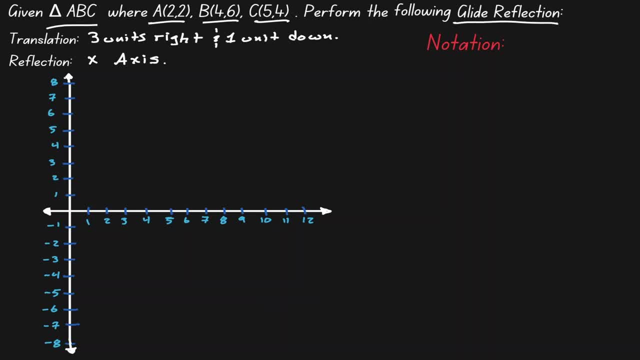 And what we want to do. we want to perform a glide reflection into this triangle. Let's start by putting this information in our plane. So, for this glide reflection, we're going to write down the reflection that we will be using. So, for this glide reflection, we want to perform the translation. 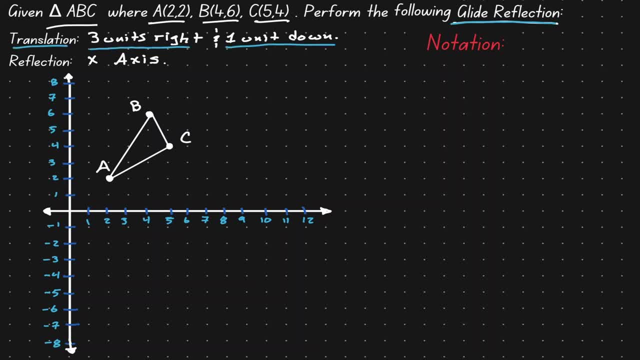 of moving three units to the right and one unit down, And then we want to perform the reflection over the x-axis. Let's start by writing this down using the correct notation. So first we want to start with the translation. So the translation for three units to the right and one unit down is capital T subscript 3, comma 1.. 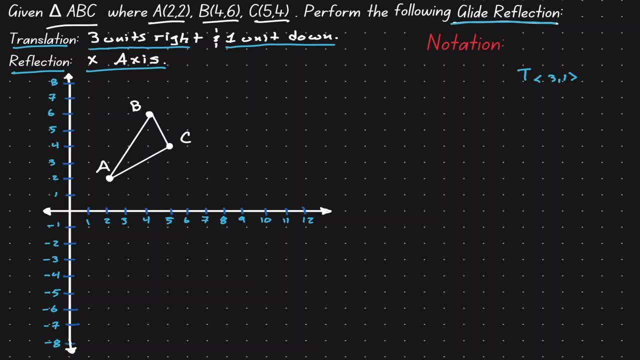 And then to indicate: then we're going to follow by the transformation of a reflection. We're going to open up a small circle And then on the left-hand side of that circle, we need to indicate what is the reflection that we're doing, which is our x-axis. 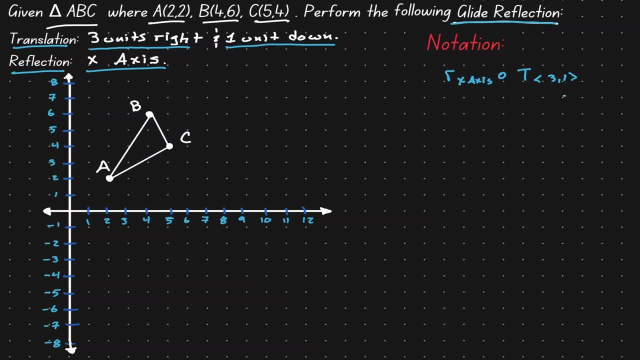 So one thing to notice is that the notation of a composition, we read it from right to left, First the translation and then the reflection. Now let's actually perform the glide reflection. Let's move every point three units to the right and one unit down. 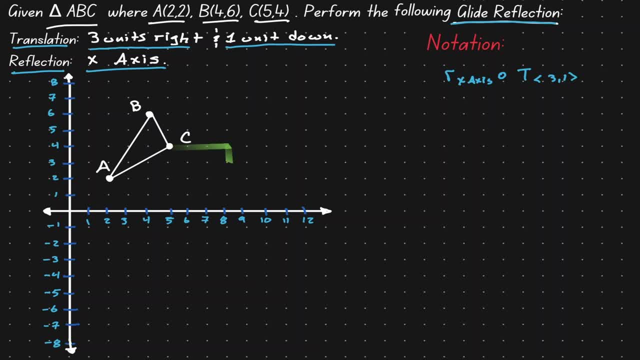 So this is going to be our location for C. Let's call it C prime. Now let's move point B: three units to the right and one down. That's going to be our location for B prime. And now let's move A: three units to the right and one down. 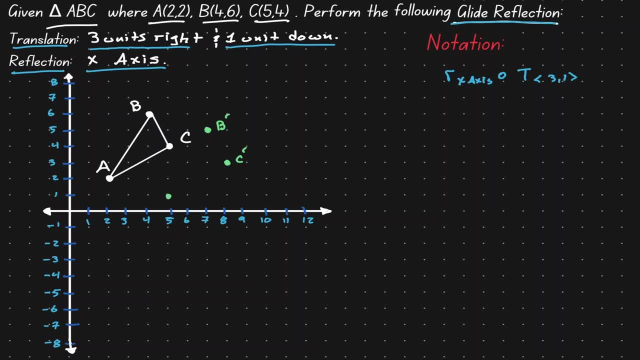 That's going to be our location for A prime. So we're done with translation. Now let's perform the reflection on the green triangle- Not on the original, but on the triangle that we got After the translation. Let's start with the point of A prime. 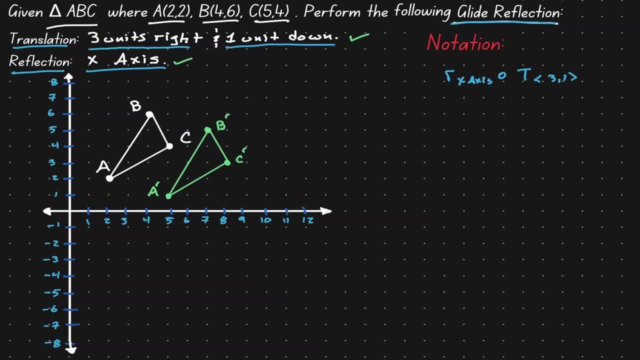 When it gets reflected over the x-axis, we end up at the location of five comma, negative one. But now to indicate that this is the location after two transformations have been applied, then we use the symbol of double prime. So now this point, we're going to call it A double prime. 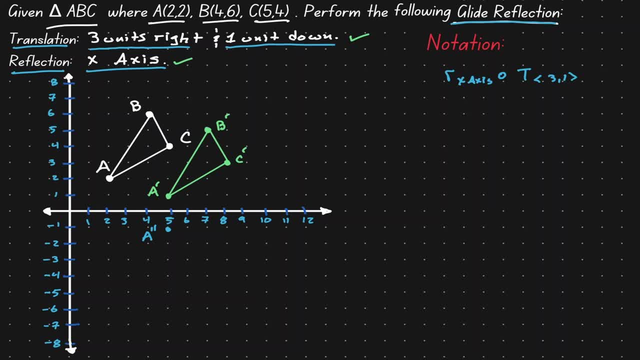 to indicate that this is the location after two transformations. So now let's perform the reflection over B prime- Our new location Will be at seven comma negative five- And to indicate that this is the location after two transformations have been applied, we're going to call this point B double prime. 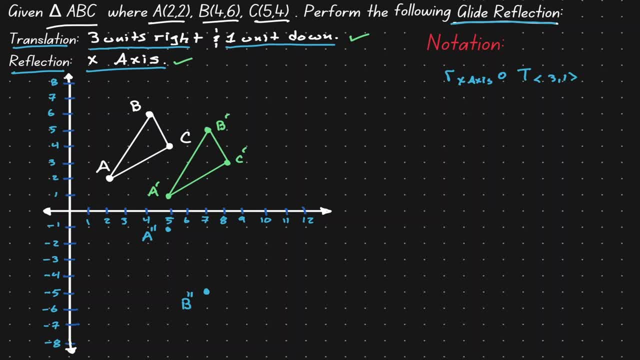 And now let's perform the reflection over C prime. Our new location will be eight comma negative three And to indicate that this is the location after two transformation, we're going to call this point C double prime. Let's connect those points And we are done. 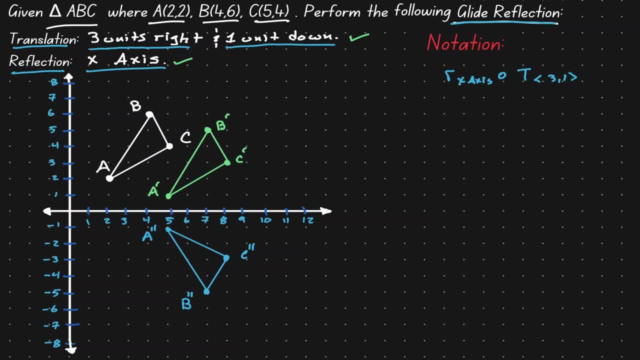 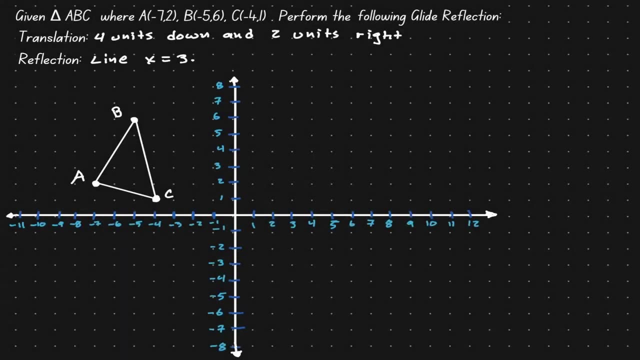 Because this triangle of A double prime, B double prime, C double prime, it is the result of a glide reflection. We first perform a translation and then we perform a reflection. Let's take a look at another example. In this example we are given a triangle ABC with the coordinate points of negative seven to. 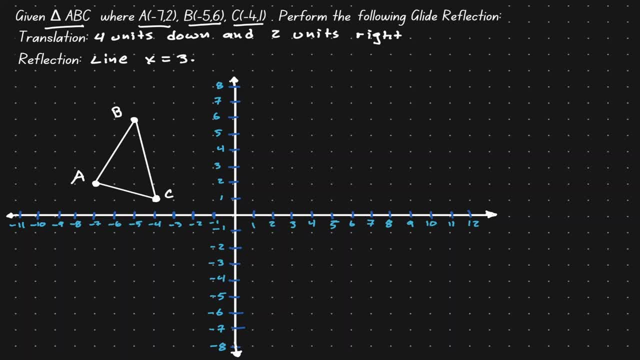 negative five, six and negative four, one. And what we want to do? we want to perform a glide reflection into it. And here we have the two transformations that we want to perform. First, we will perform a translation of four units down and two units to the right. 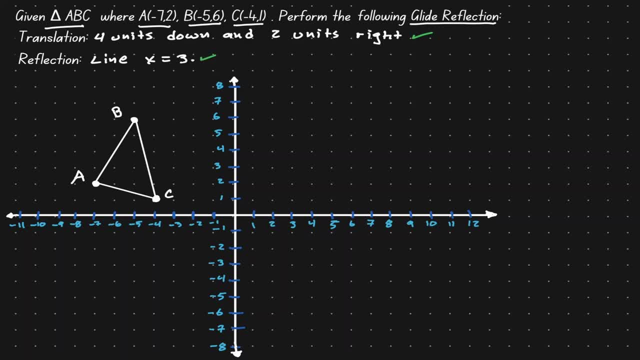 And then we will perform a reflection over the line x equals three. So let's write this down using the correct notation. First is the translation of four units down and two units to the right, And then we follow with the transformation of a reflection over the line x equals three. 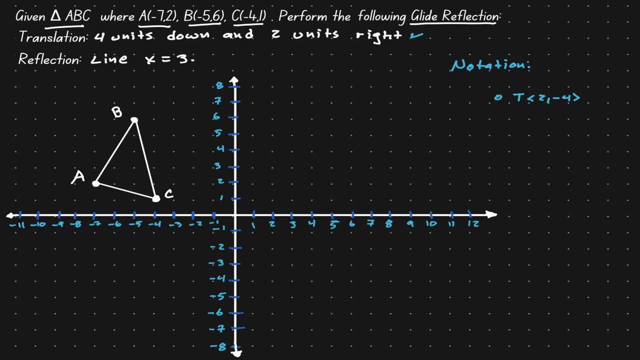 To follow the notation, we're going to open up a circle And then, on the left hand side of it, we're going to write down our second transformation, Which, in this case it's a reflection over the line x- equals three, And let me remind you that the way that we read this composition function. 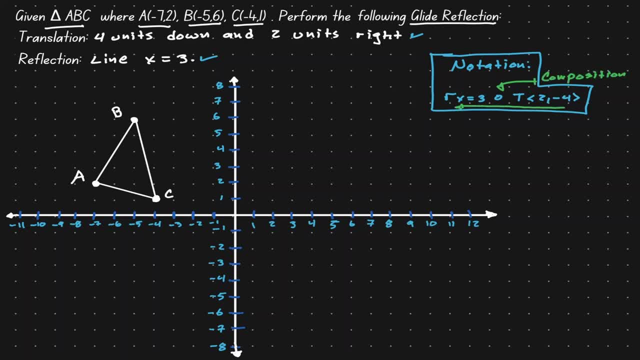 It is from right to left, First the translation and then the reflection, Always right to left. Let's start with point C. let's move it 4 units down and 2 units to the right. After that movement we have a location: a negative 2, negative 3.. 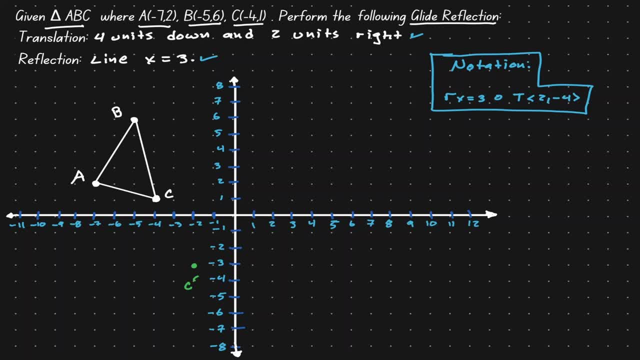 So let's call that C' Now. let's translate point A: 4 units down and 2 units to the right. Let's call this point A' Now. let's translate point B: 4 units down, 2 units to the right. 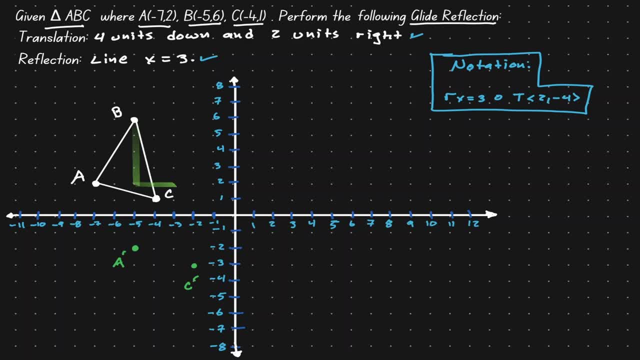 We're going to end up at the location of negative 3, 2.. Let's call this point B' Now let's connect those points. So now to perform our glide reflection. let's reflect this green triangle over the line x equals 3.. 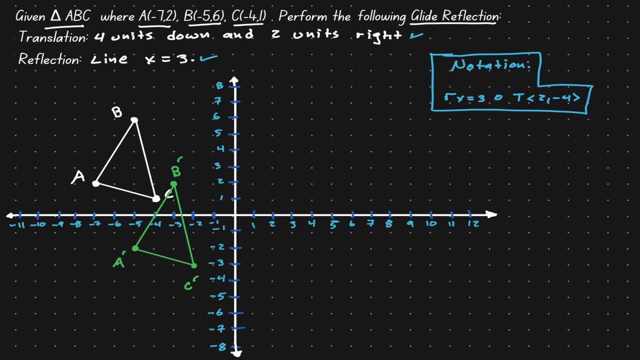 So let's start by drawing our line x equals 3.. Again, it is a vertical. It is a vertical line passing through the point of x equals 3.. Let's start by reflecting the point C' Notice that C' is 5 units away from the vertical line. 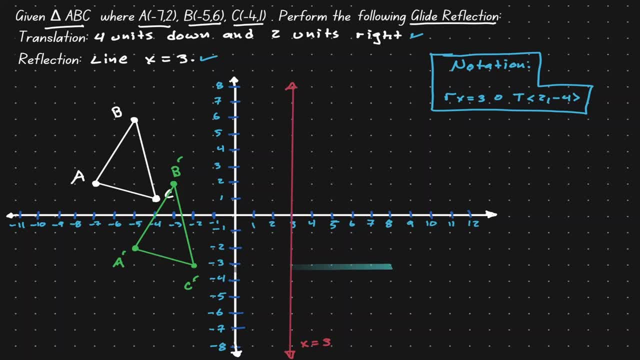 So notice that after the reflection it should be 5 units away from the vertical line as well, on the opposite direction. So we end up at the location of 8, negative 3.. Let's call that point C' Notice that in this location. 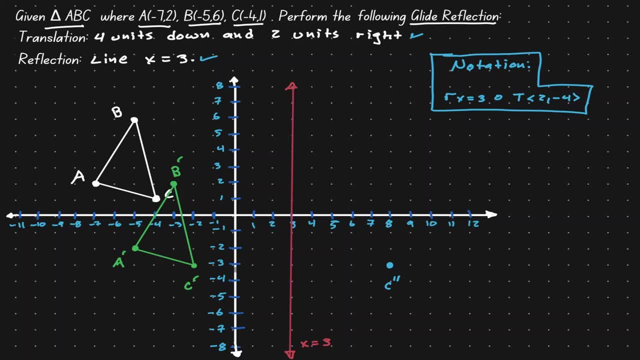 we have to do. we have to do a double prime, because this is the location. after two transformations have been performed on point C. Now let's reflect point A' Notice that it's 8 units away from the vertical line. So after a reflection, 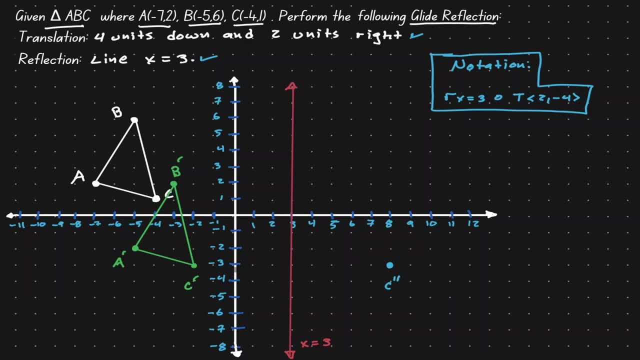 it should be 8 units away from it as well. So we end up at the location 11, negative 2.. Let's call that point A''. This is the location of A after two transformations have been performed to it. So now let's reflect the point B'. 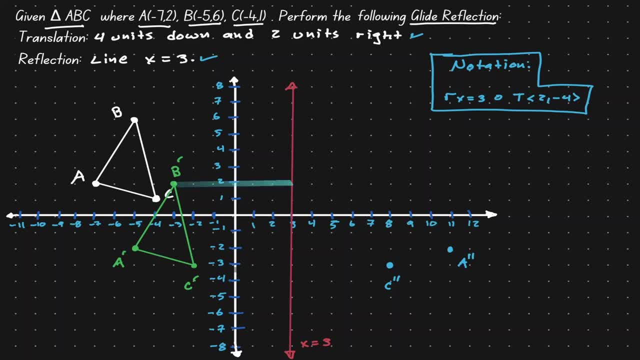 So now let's reflect the point B'. So now let's reflect the point B'. It is 6 units away from the vertical line, so after a reflection it should be 6 units as well. So we end up at the location of 9, 2.. 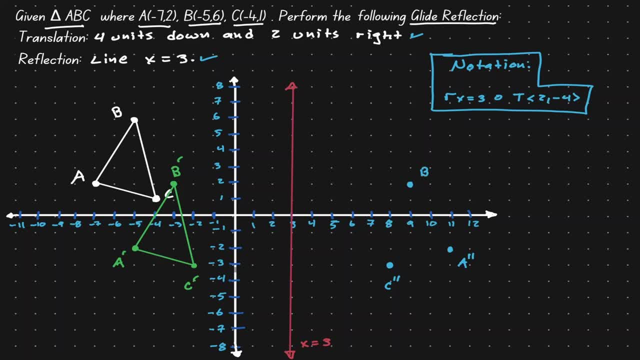 Let's call that point B' This is the location of B after two transformations have been performed to it. So now let's connect those points, And here we have our final result: Triangle A'B'C' Triangle A'B'C'A'B'C'A'B'C. 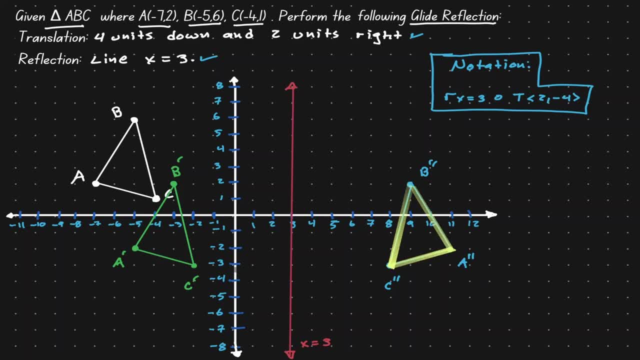 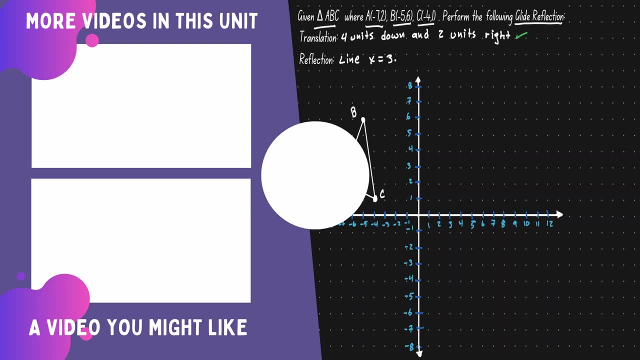 Triangle A'B'C'A'B'C'S'A'B'C'A'B'C'B'C'A'B. It is the result of a glide reflection on triangle ABC. Hello, if you would like to continue learning about mathematics, you can check out the videos on the left.